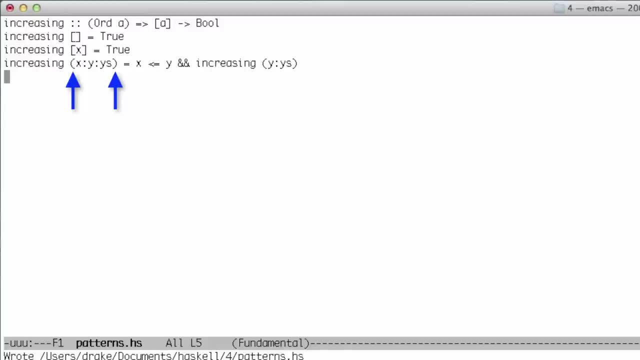 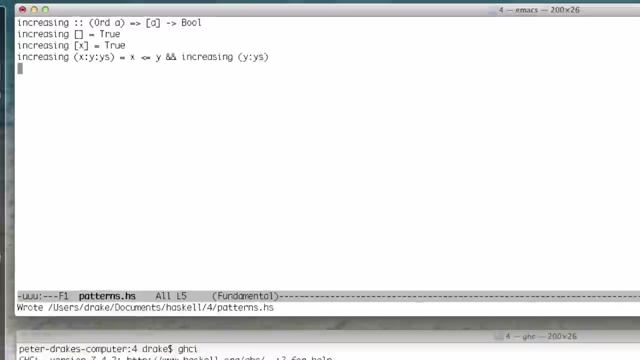 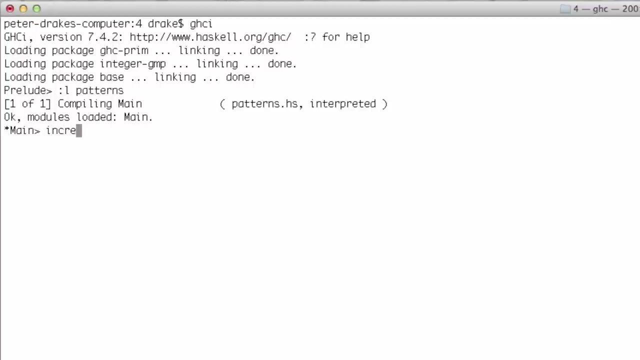 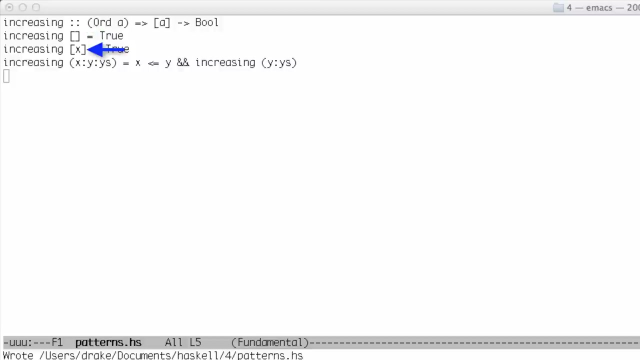 We can add and subtract, as a guide, several things at once. In evaluating a call to increasing, Haskell goes through the list of patterns until it finds one that matches. For example, if we ask for, The first pattern doesn't match but the second one does, with x being 5, so the expression 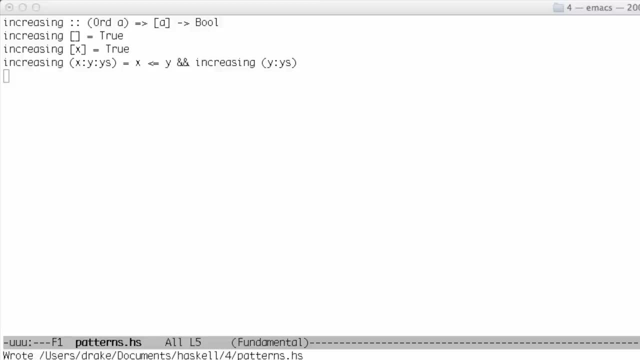 evaluates to true. Since Haskell goes through the patterns in order, we can be even more concise. This handles the case where the list has at least two items, then says that any other list is increasing. The underscore matches everything. For clarity. we use this when we don't care what we matched. 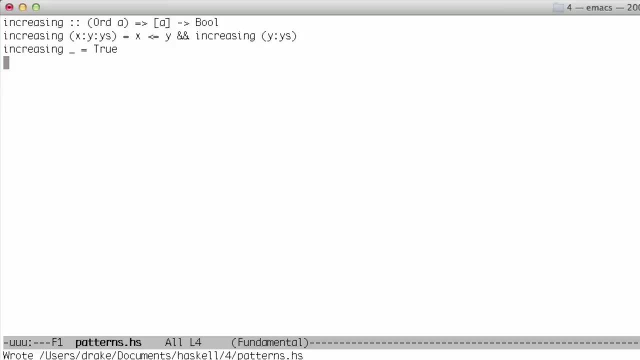 Here's a function that takes a string and returns the same string with no vowels. This says: if word is the empty string, just return it. Otherwise, if the first letter is a vowel, return the rest of word without vowels. If it's not, return the first letter plus the rest of word without vowels. 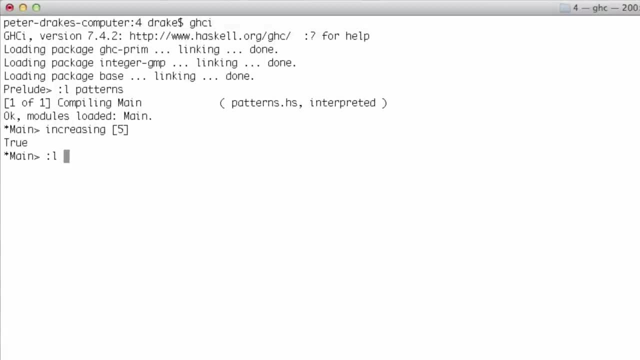 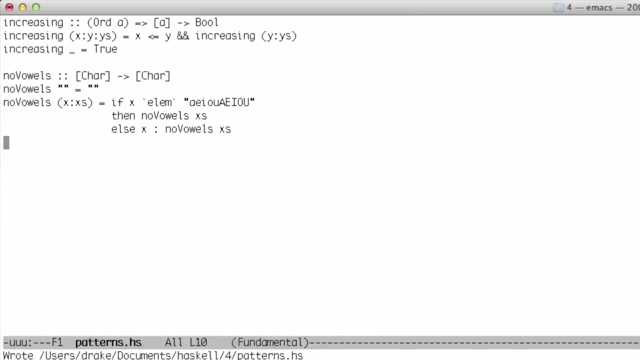 Let's give it a try Here it is with. with pattern matching. We don't have to constantly use head and tail to take 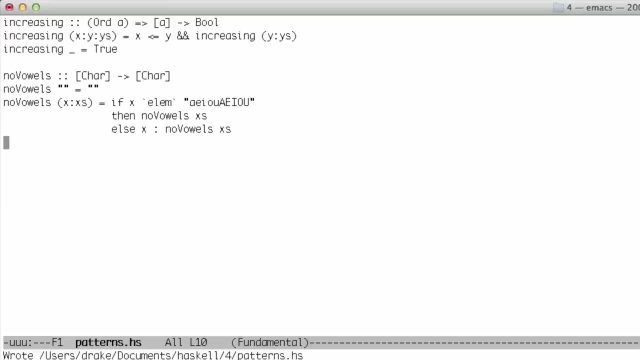 apart the word, because the pattern matcher has already broken it down into X, the first letter, and X's the rest of the word. We can also use guards to specify a series of conditions and what we should do in each case After each. 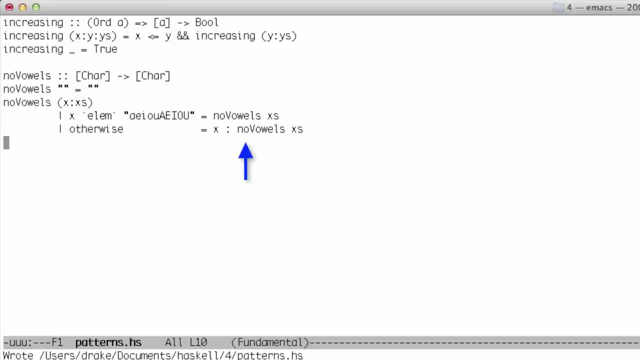 vertical pipe is a Boolean condition, an equal sign, and what the function returns. in that case We only have two conditions, including the default, otherwise here, but we could have any number. This is analogous to a cond statement in Lisp or Scheme. Our next function calls out the report of the 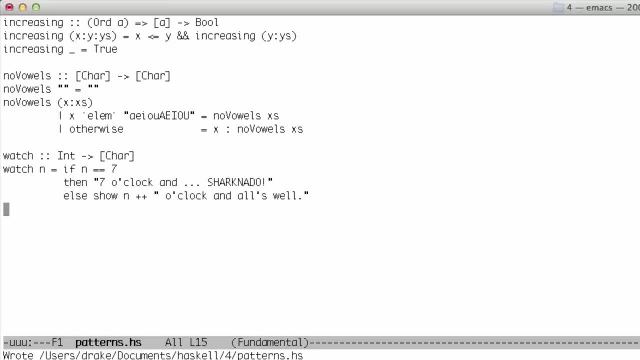 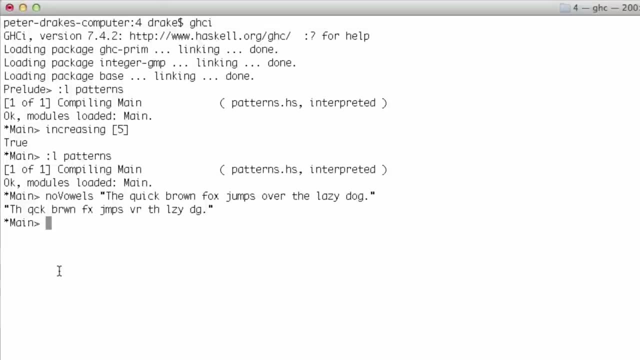 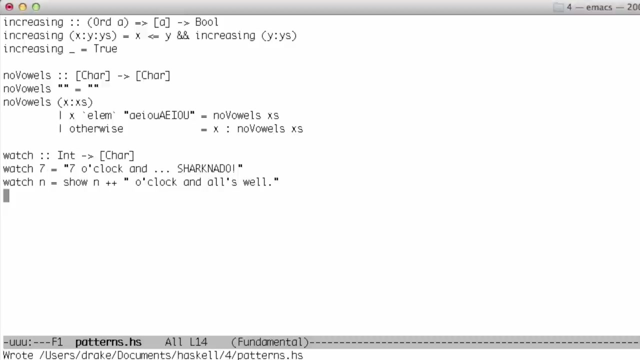 night watch. Occasionally there's cause for alarm. The show function converts the int n into a string. Let's try it out Here. it is with pattern matching. We can avoid a small amount of redundancy by using a where expression. This gives a single expression, then defines the. 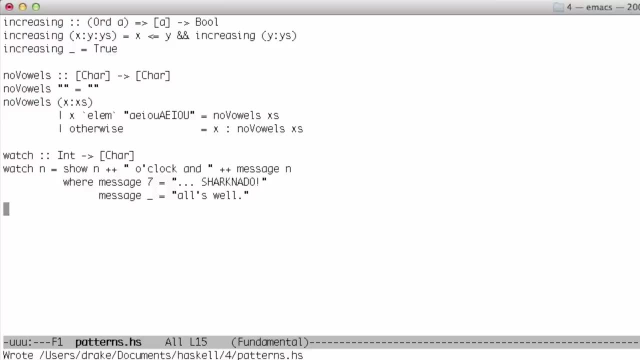 function used in that expression. Is this clear In this situation? it's a matter of taste, but sometimes one version will be significantly more concise. Yet another way to write this function involves a case statement, which is like a switch statement in C or Java. 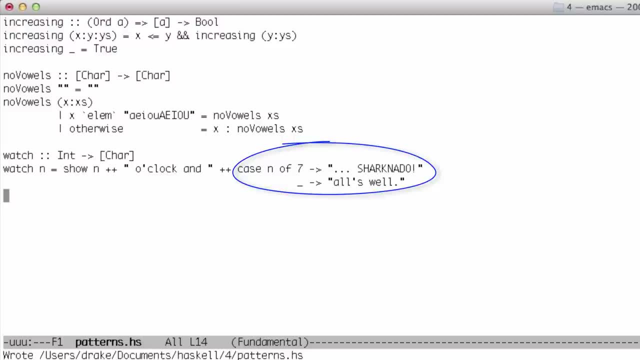 This lists several possibilities for n, along with a value for each one. Again, an underscore matches anything. Here's one last function which calculates the acceleration due to gravity at distance r from the center of the earth. The first mysterious number is the universal gravitational constant, The 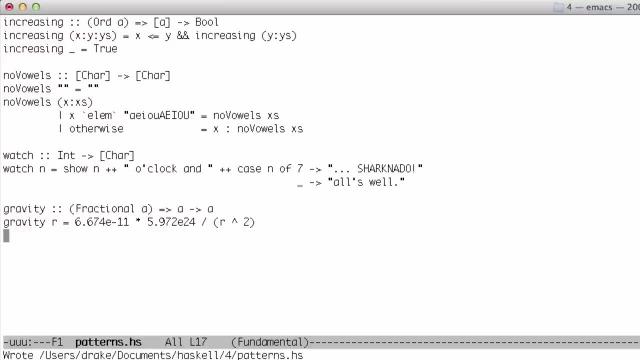 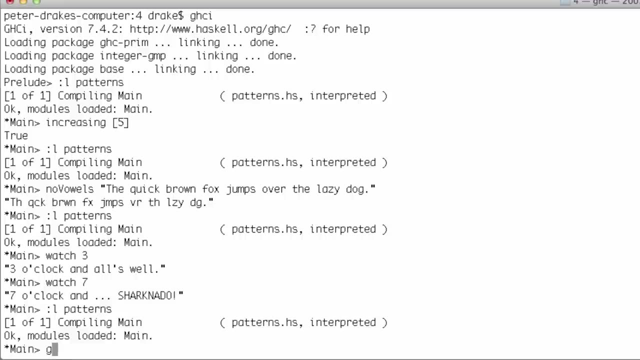 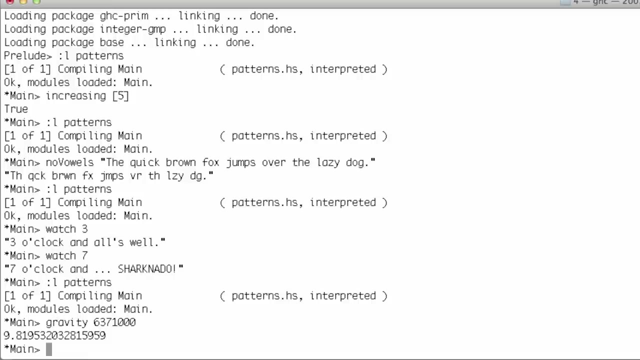 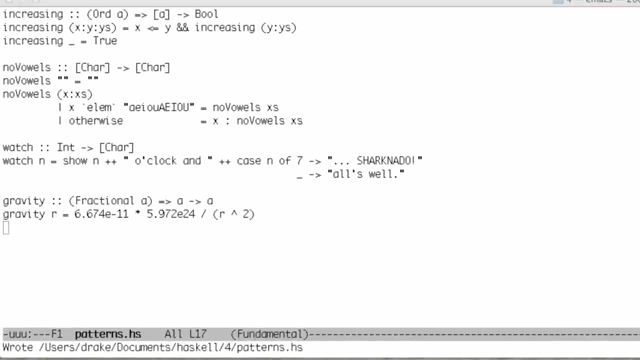 second one is the mass of the Earth. We can test this function by passing it the radius of the Earth. That's about right. The function would debatably be clearer if we gave those constants names using a let expression. We couldn't have just defined these as global constants. on. 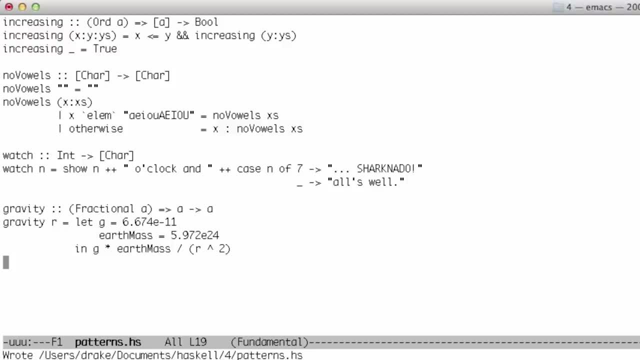 separate lines. The advantage of let is that the binding is only visible within the scope of the let statement. Good names are hard to come by, so it's better to define things as locally as possible. Examples are good, The best way to learn. 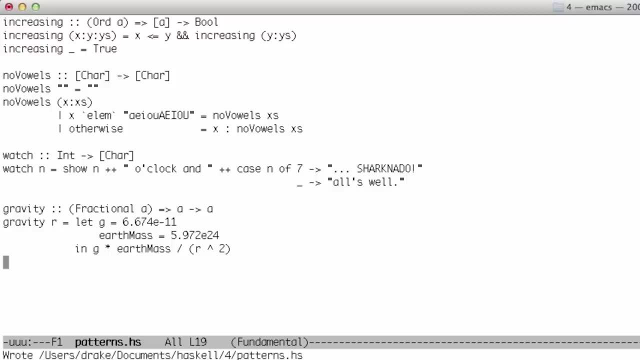 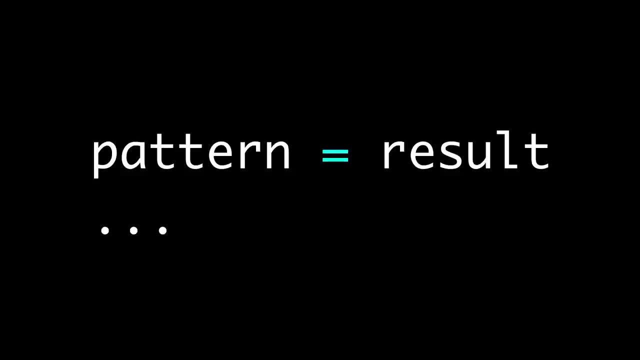 is to solve more problems using these techniques. If you prefer explicit rules, though, you might appreciate some templates. A definition looks like this: It's okay to list several different patterns involving the same function name, as we did with increasing. The patterns should be exhaustive so that no.